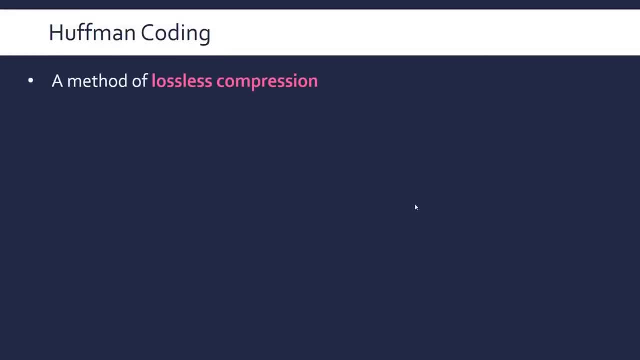 Hello, this is going to be all about Halfman Coding, which is a method of lossless compression, So two key topics that are relevant to this video are ASCII and representing text in binary, and actually representing images in binary as well, and, of course, the compression video. 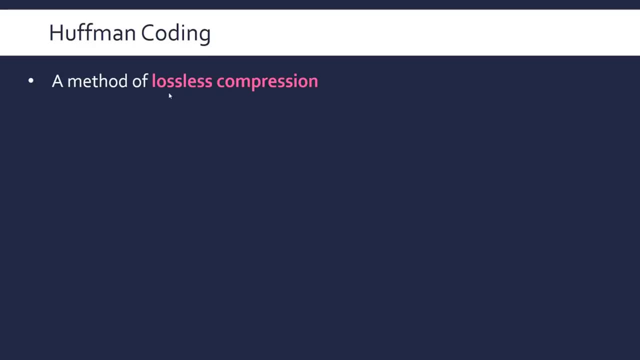 about lossy and lossless compression. So Halfman Coding is a way to reduce the size of usually text or images without losing any of the actual data. And the whole principle of this and the reason it works is because some data in a file is 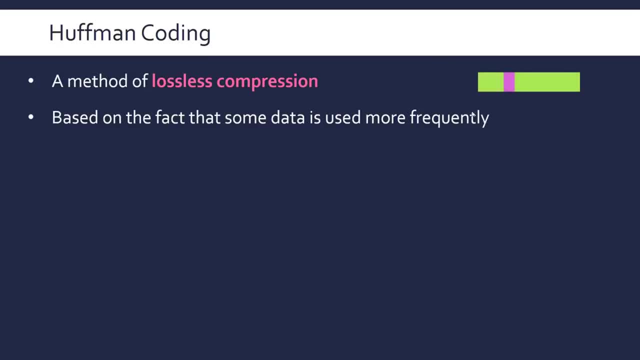 used more frequently than others. So some colours are used more often in an image, like green here is used more often than purple, and in text some letters are used more frequently, like A is used a lot more frequently than Q, for example, Using standard representation, like with ASCII or bitmap images that we looked at each piece. 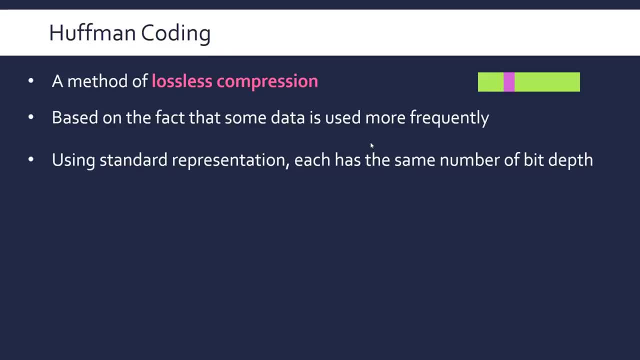 of data, like a character or a colour, has the same number of bits as all the other characters or colours, So there's no flexibility here. they have what's known as fixed length encoding, ie the bit depth, the number of bits assigned to each unit. 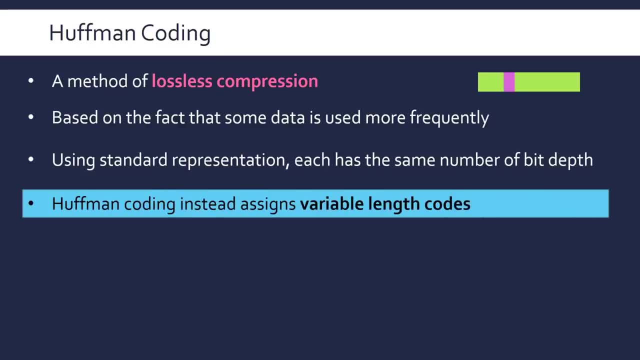 is the same regardless of the unit. So with Halfman Coding we can instead assign variable length codes so we can have different bit depths for different pieces of data, And to tie this together, the more frequently the character or colour as well. we're going. 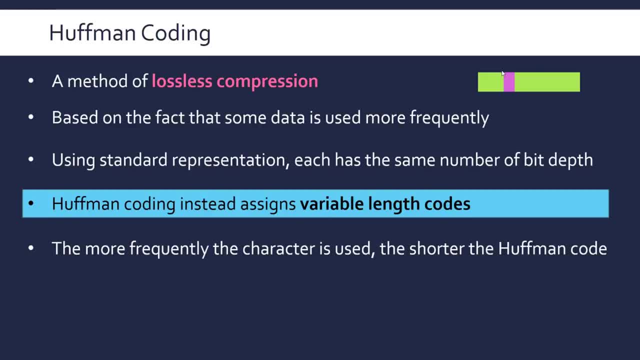 to look at text in this video, but it's the same process for images. more frequently the piece of data is used, the shorter the Halfman Code will be for it, so we can reduce the total file size as much as possible. we want to minimise the file size. 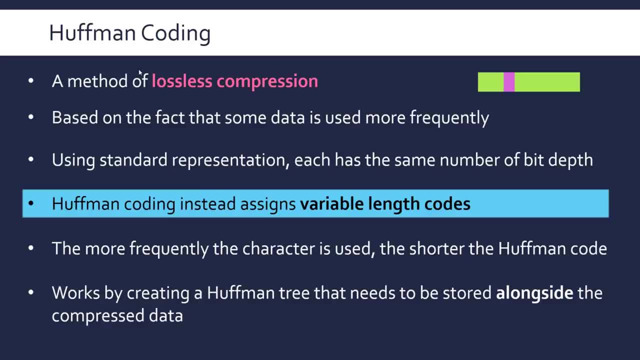 So the actual process, the algorithm that produces a Halfman Code for each character, works by creating what's known as a Halfman Document. It's a tree, a binary tree that's stored alongside the compressed data. so that is quite important, but we'll go back to that after we look at the algorithm. 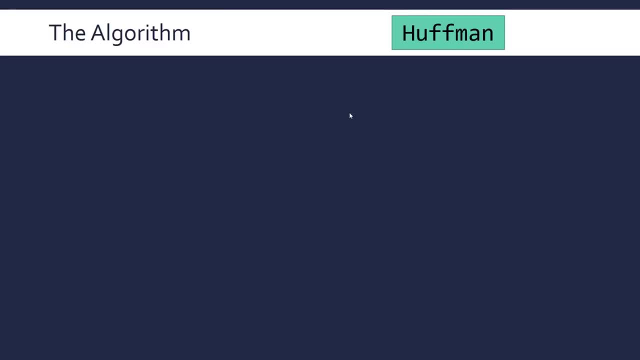 So, before showing you the steps, we're actually going to implement this with Huffman, just a single word. obviously it would be much, much longer with a whole text file, but for simplicity's sake it can get quite complicated, so we're going to start with just a single. 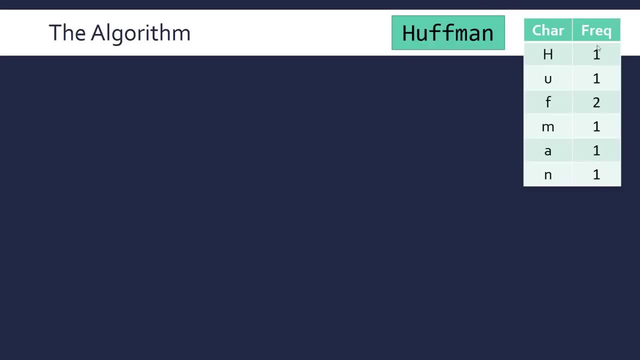 word and we've got. if we look at the characters and their frequencies, remember uppercase is different to lowercase and you can also have spaces as a character. but we can see we've all got one frequency apart from f, which is repeated twice. But anyway, we'll leave this for a second. 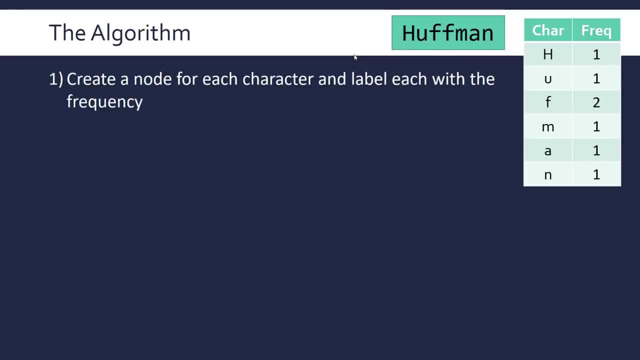 Let's talk about the general abstract steps. So first of all, we need to create a node in our graph for each character and label, each with a frequency. We then have to arrange these nodes in ascending frequency. We're then going to take the first two nodes and join them, which basically creates a new. 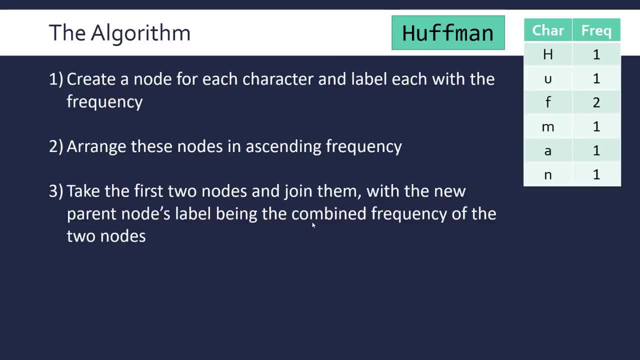 parent node and we have that label being the combined frequency of the two nodes. We then need to kind of reinsert this node with the two children attached back into our ordered list, so make sure it's still in ascending frequency. and then we have to repeat these. 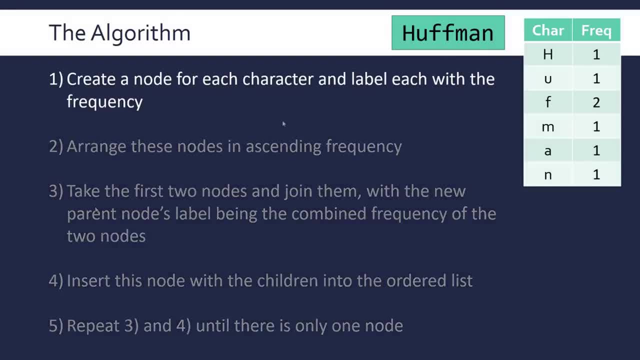 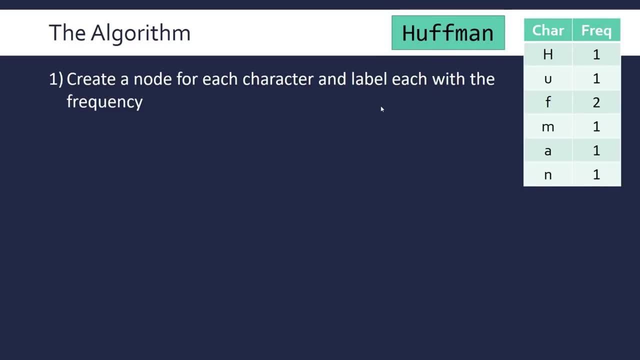 two steps until we reach an actual tree where we have a root node. Let's step back then and actually implement this with Huffman as our single bit of text, and the process is the same for images, but often text is more frequently used up because you're kind of forced to use loss as compression with text. 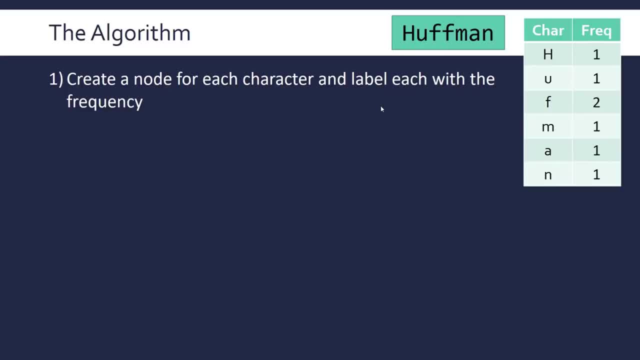 You can, with images, throw away some of the data and just lose a bit of quality. but with text you have to retain every character, otherwise you lose just the whole meaning of your text. So first of all we need to create a node for each character and label each with a frequency. 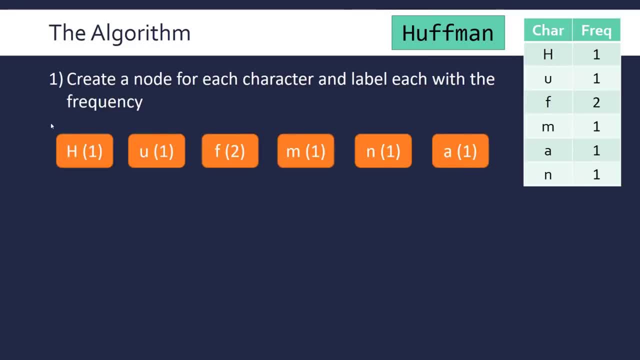 You may not really come across graphs before if this is the first time you're doing this, but a node is just kind of a single unit. You can do a circle, a square, it doesn't really matter, And usually we label it with our character and then the frequency in brackets. other 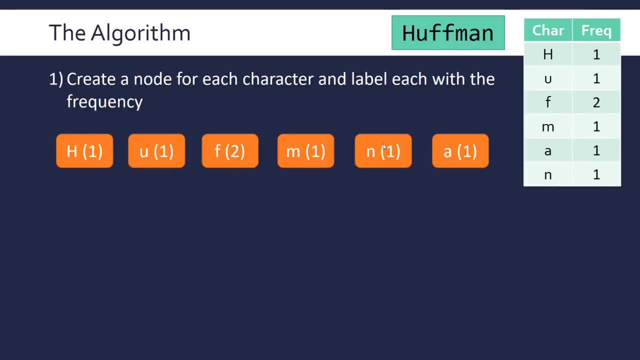 way around is fine, just as long as you're consistent. So you need to basically show both the character and its frequency from the original text, like we've done here. Okay, so this isn't in order. you can see we've got F here, so we need to put it in ascending. 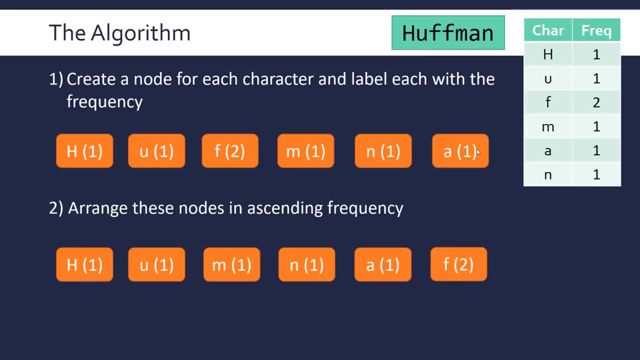 order. so the two goes to the end, And this is where the actual implementation can change, depending on how you're actually going to code this, perhaps. So I've just shifted it to the end, but the order otherwise is saved. You've got to kind of think how a sorting algorithm would do this, but this is an added 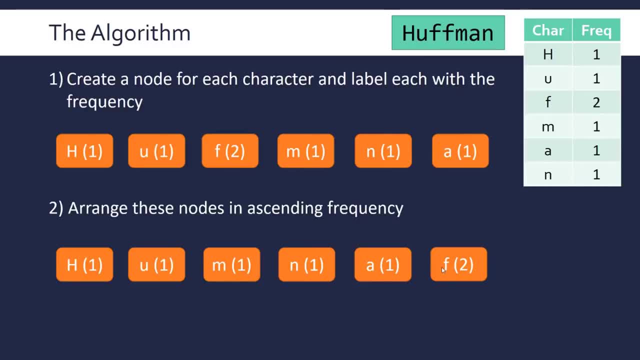 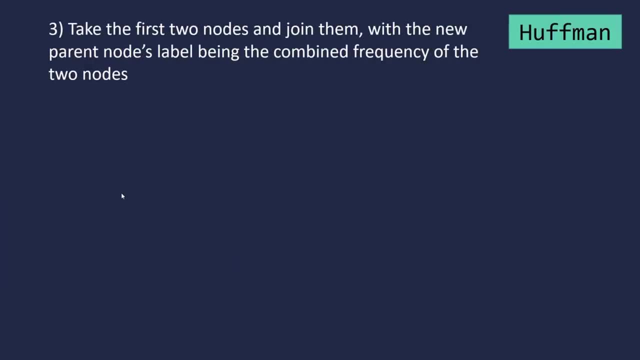 complication. we don't have to worry too much when we're doing it by hand. So basically we've got our nodes separate, but in ascending order. In this order, the first two nodes are H and U, so we need to then basically combine them and make a parent node. 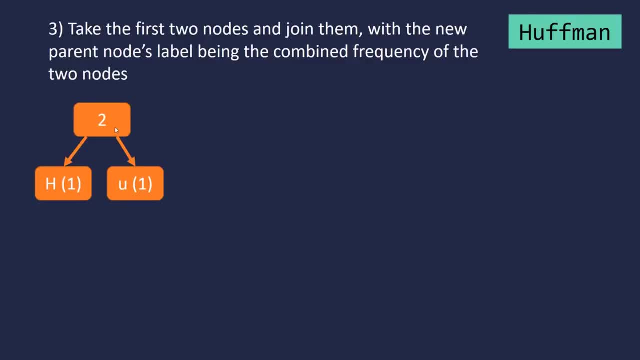 So we basically will draw this. so we've got H and U connected with a parent node, and this parent node hasn't got a character but it's just got the combined frequency of its children. So 1 plus 1 is 2.. And then we have the rest of our other nodes which haven't been done. 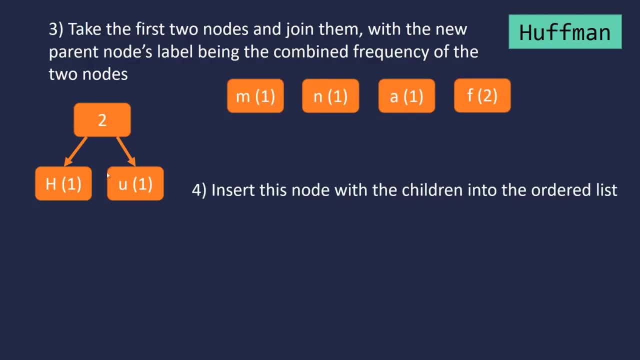 They haven't joined yet And basically we need to re-insert this back into our list. so we've kind of taken this away and we need to put it back. making sure the order is the same. So 2 is now going to be compared to the other frequencies here. 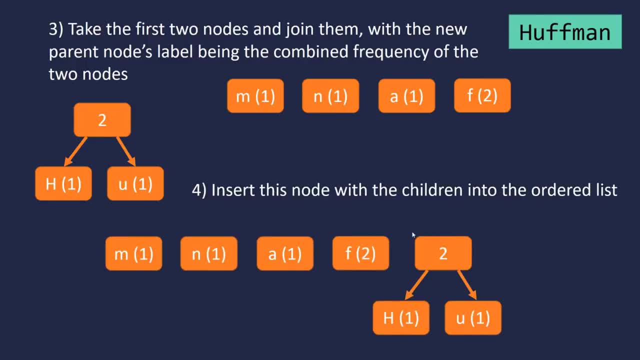 So again, we can kind of just put it to the end. we've now got two 2's, but again for kind of, if you put it in between A and F, your actual result would be different, but it would still be correct because of just the nature of this coding. but we'll talk about that a bit later. 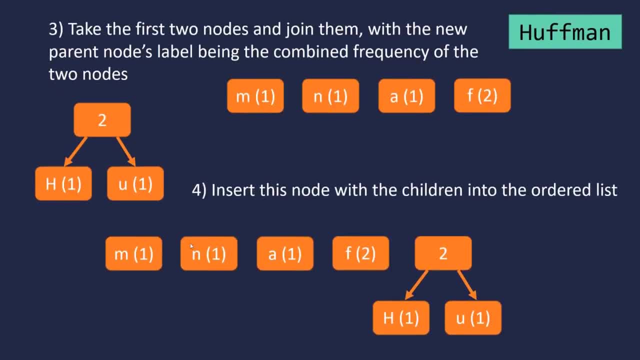 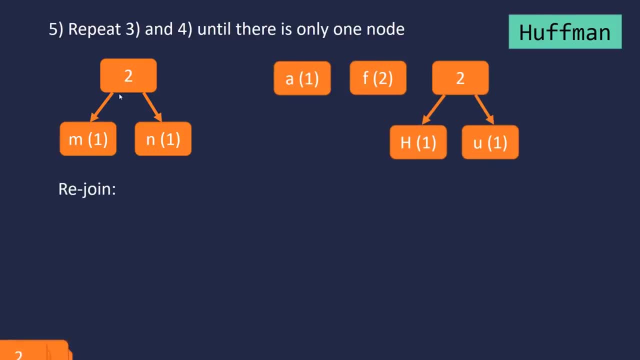 So now we need to again just do a couple of repeats. so our first two nodes are M and N here, so we need to combine them and add their frequencies very similar, then re-attach it to our list. The next two smallest nodes are now A and F, so we need to combine them. 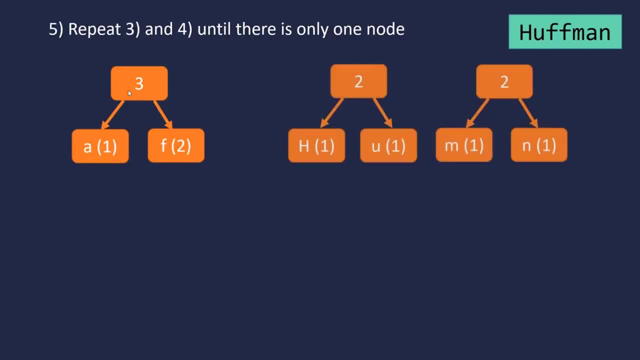 So the two frequencies, 1 plus 2, is 3, and then we have to re-insert this to our list. Now it's exactly the same. we've still got to combine our smallest two nodes, so we're kind of working at this level. now this is kind of a sub-level, so we're now just looking. 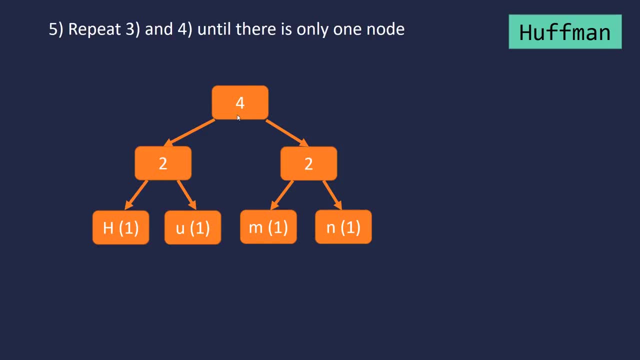 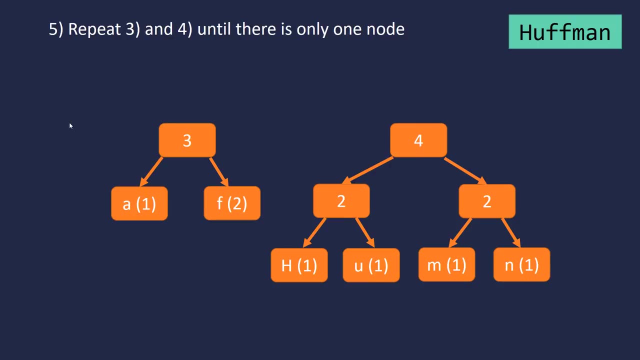 at 2 and 2, so we've got to combine those. Our parent is going to be 4 and we still have the other one And we need to order this, so 4 goes to the other side. We need to combine 3 and 4, 3 plus 4 is 7, and so we finally have a root node. we've only 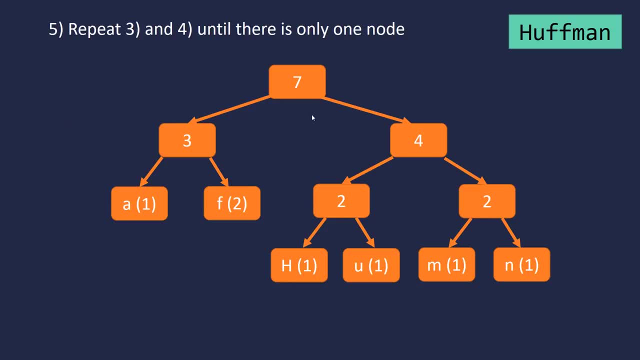 got one node. all the other. well, we've only got one root node. all the others inherit from this and a good way to check is that the top node should equal the total number of original characters. so we've got 7 characters in Huffman, we've got 7 here, so they do match. so that's. 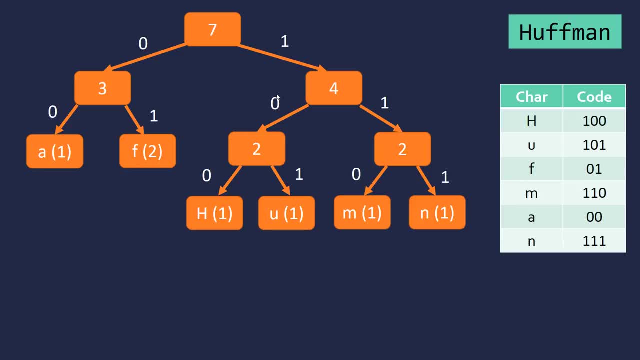 good, And there is one final step, which may be implicit depending on the implementation, but we need to label our arrows, And so we're going to say that the left arrow is going to be 0.. And the right arrows are going to be 1.. 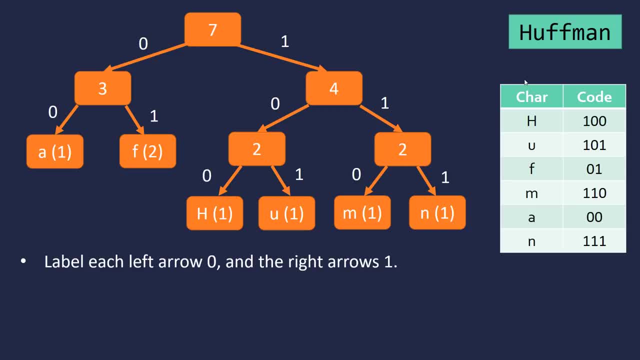 And it could be the other way around. it doesn't actually matter, the codes would just be the opposite. but convention is usually left is 0 and right is 1.. So to actually get the codes here, you can see I've magically filled in this table. 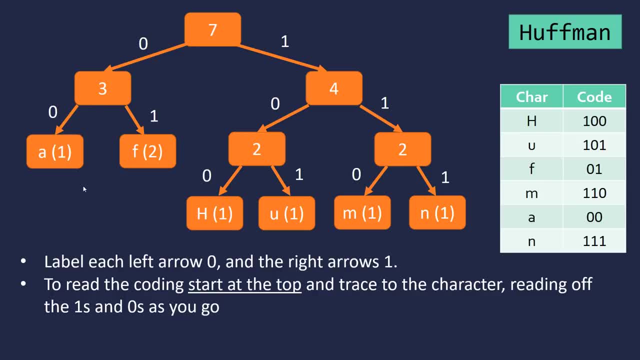 We need to start at the top and trace to the character so you can see all our characters are at the bottom, so they're in the bottom levels, which is a good sign. It would be a bit of an issue if they weren't. So the idea is, if you want to find out what H is, we locate H on our tree and we go ok. 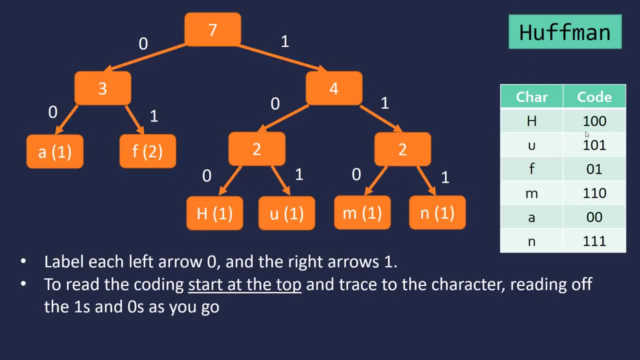 so it's going to be 1. 0, 0 and that's our code for H and for U it's going to be 1: 0, 1, like here. for F is going to be 0, 1, like here. and basically the idea is you follow the tree using the labels until 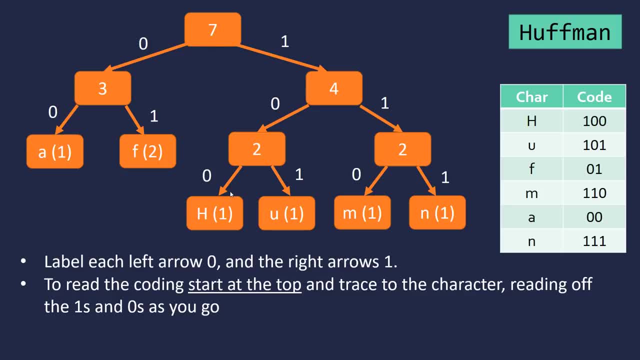 you get your character and that is going to be the code. so it's going from the top to the bottom and that's how we're going to do it. It's really important to say the Huffman codes are specific to the text you've used, so Huffman. 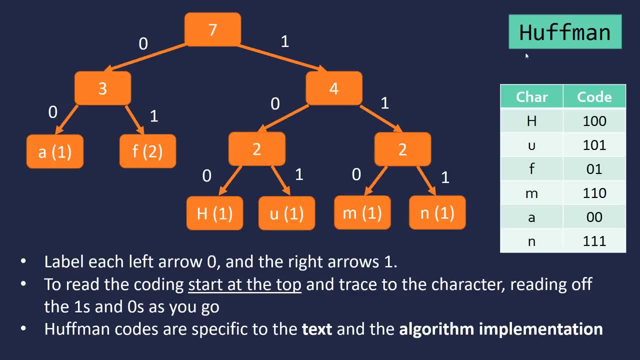 in this case and also the algorithms implementation. So if we'd used Huffman coding as I said, So if we'd used Huffman coding as I said, We would get different codes. potentially or definitely we'd get different codes. and if I made other decisions when I was doing the algorithm, like the order, if I changed? 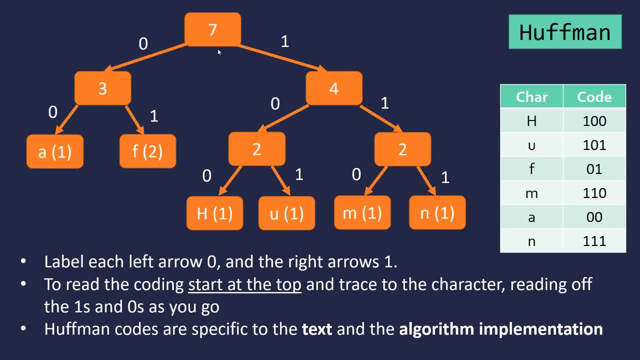 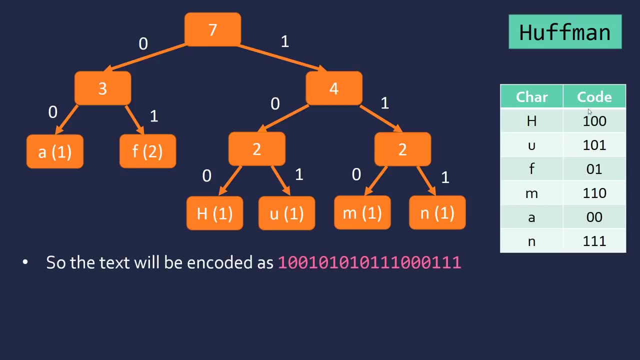 the order up or left equals 1, right equals zero, we'd get different codes. So these codes are specific to how you've actually done the algorithm and that's fine. the whole idea is they are tied to this tree. So actually compressing this if we combined these codes together, so 1 0, 0 following them. 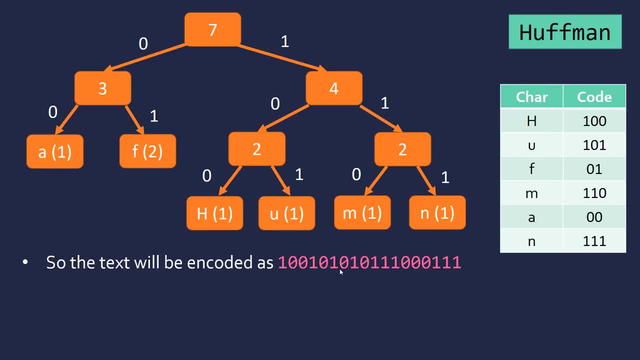 we've got to make sure we have two F's in the middle here, so we've got 1 0, 1, 0 for two Fs. If you just concatenated all of these together to form Huffman, this is the long binary string we'd get In order to extract the characters. to decompress the text: the. 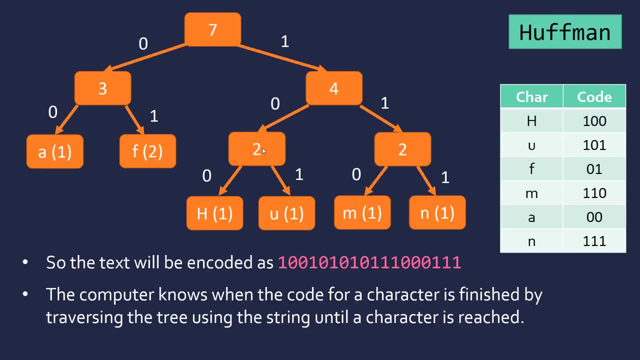 computer will use the tree It knows when the code for the character is finished by transversing the tree using the string until the character is reached. Here there's no way inherently to know if 100 is a character or 1001 is a character, so we need to use 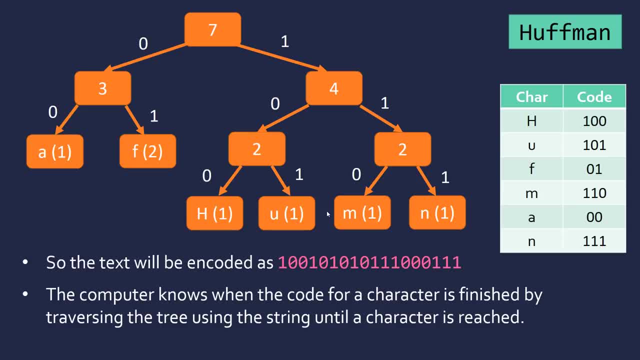 the tree to find this out. In ASCII, it knows that every single value equals a single character. It will count to seven and then use that as a character, Whereas here they're variable lengths. We don't know how long it's going to be, unless we use the tree as well. 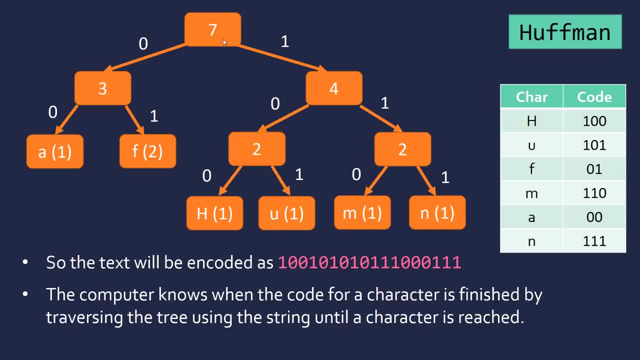 What it will do. it will start at the top, look at the string and go 1, 0, 0.. The first three are going to be H, because we've reached the bottom level of this tree. We can't go. any further. The first three are definitely going to be H. Then it will go: 1001, 1002, 1003, 1004, 1005,, 1006, 1007, 1008, 1009, 1009, 10010, 10010, 10011, 10011,. 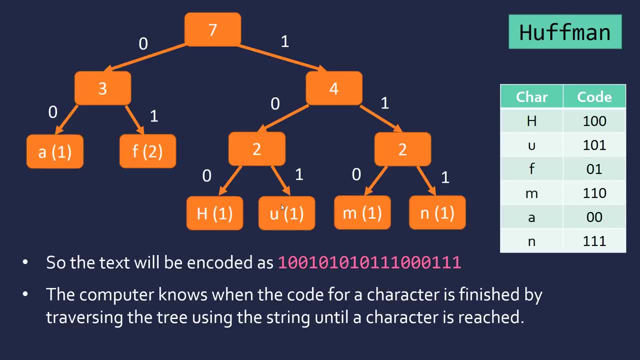 10012, 101 for U. Again, the next three are going to be U, because we can't go any further. We're using the tree to actually work out where this comes from. We're doing the same process we did before, where we traced down to actually find the 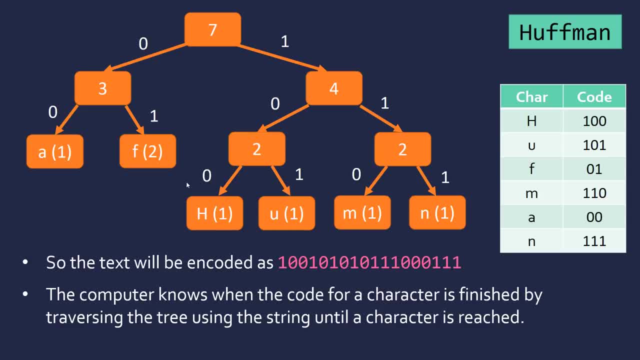 code. That's how it knows when a character is finished because it's reached the bottom level of the tree. Really important. you understand. this is feeding the string through the tree to actually extract the characters. It's using the tree alongside the data. This is the data. 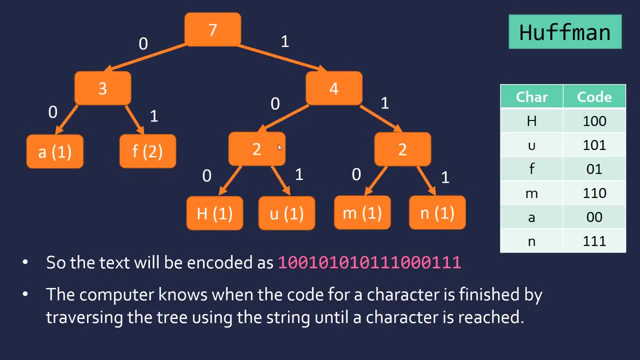 and this is the tree. They need to be stored together in order to decompress the text. Without the tree, this binary string is meaningless. No one could interpret it, and so we need the tree alongside it to give it context. To look at the effect of this. I've got the characters here. I've got F in bold because 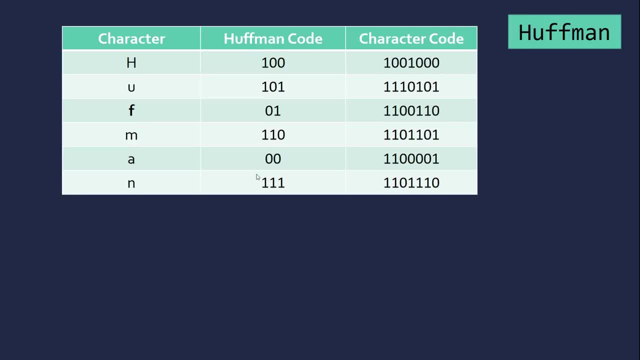 we've got two of them. just to remind you that we've got two. We've got the Huffman codes we've just worked out. We've also got the character codes for ASCII. For ASCII, this is normal ASCII, so seven bits per character, Clearly. first of all, these are a lot longer. 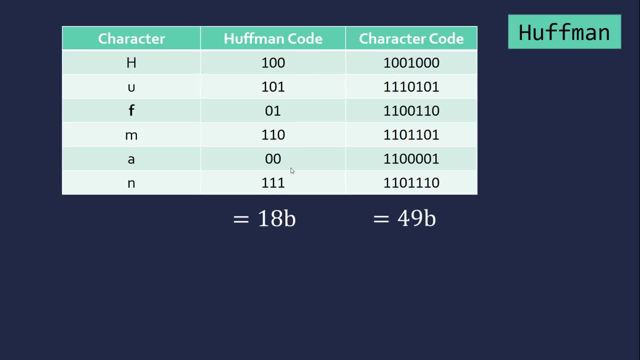 than the Huffman codes, which is not good for our data storage. This is 18 bits in total. if we count F twice, This is in total for the character codes, so 49.. Seven times seven, seven characters times seven bits per character, To work out what's been saved, we do 49 minus. 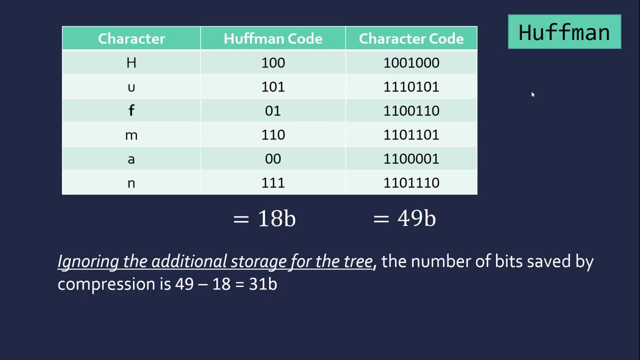 18 and that's 31 bits. we've saved Not a big deal. It does demonstrate the difference. but if we had a very long bit of text, this is going to be significant. We are ignoring the additional storage for the tree. We've got to store the tree, but we don't know how. 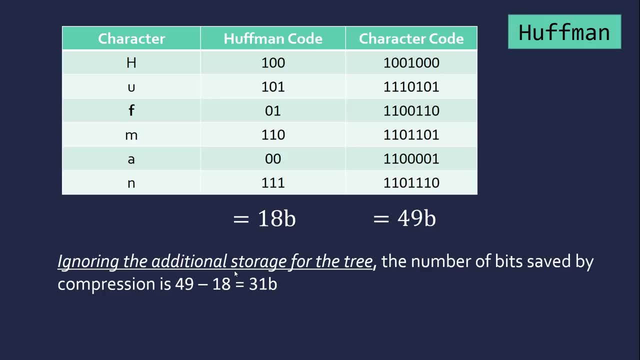 big that's going to be. It does depend on various factors which you can't know just by looking at the codes. It may have some effect on a small level, like this, but on a very large level, like a page of text, it's not going to have much effect. 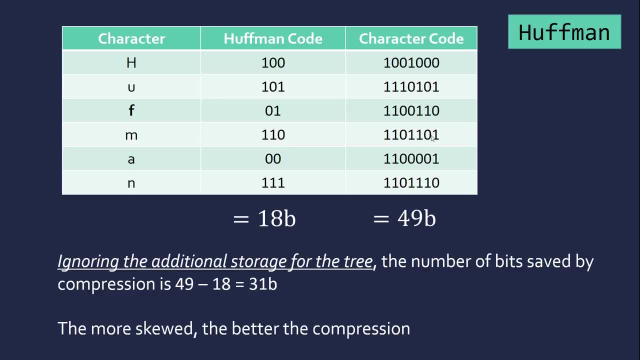 Just as a final note: the more skewed the data is, the better the compression is going to be. Hopefully you can see that If we have data that is skewed very heavily towards one character- ie one character is used a lot more often than another character- then 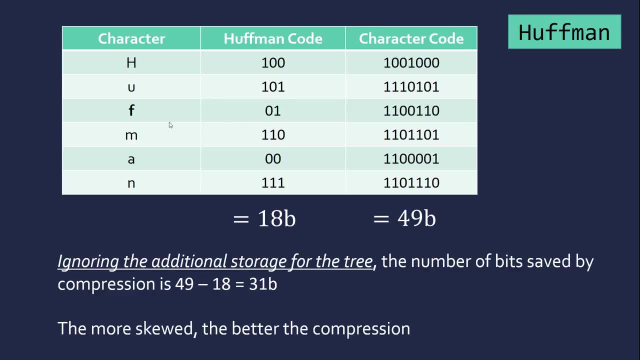 we're going to have a good compression rate because we are minimizing the storage for that character, and that character is being used a lot. That's perfect. If we have an even distribution, ie every character is used the same number of times, we may still.